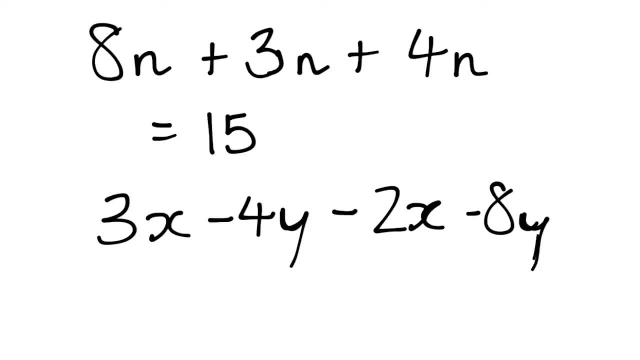 of n plus 3. lots of n plus 4, lots of n. That means I have 15 lots of n. The next one In this one I have 4 terms. The first term is 3x. the second term is minus 4y. the third: 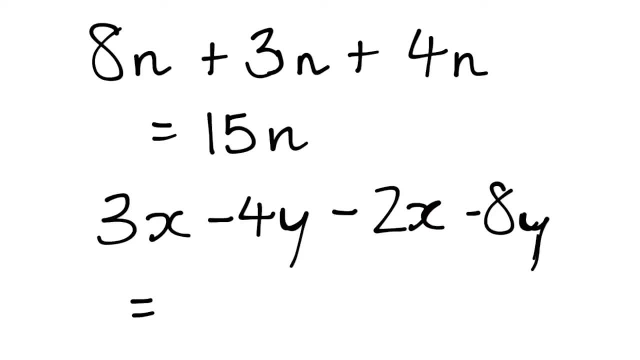 term is minus 2x and the fourth term is minus 8y. Now, in the first one, all of those terms were what we call like terms, because they all had the same letter. In the second example there were 2n. 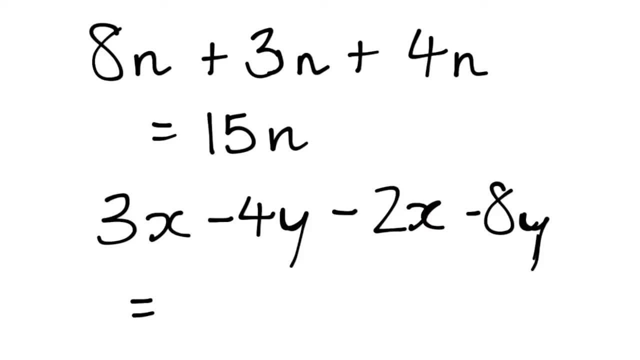 There were 2 different terms, one with x's and one with y's, And we can only combine like terms, In other words the letters that are alike. So for 3x and 2x, I'm going to circle those, And when we circle the terms you need to make sure you include the sign. 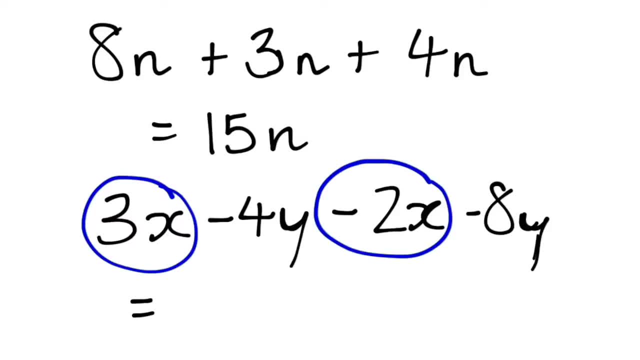 in the term. So the 3x would have a positive sign in front of it. if there was a sign there And the 2x has a minus sign, I need to circle that minus sign because that belongs to that 2x. That's making that 2x a negative. So to combine those two terms I'll have 3x minus. 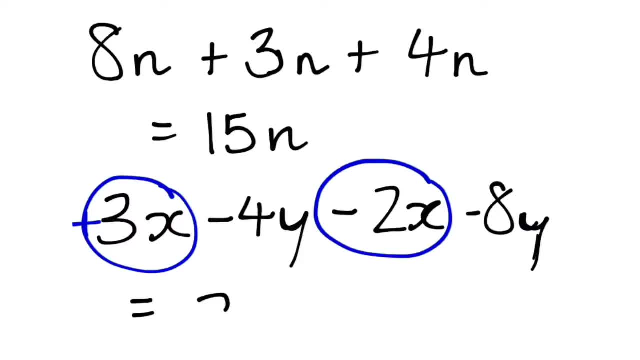 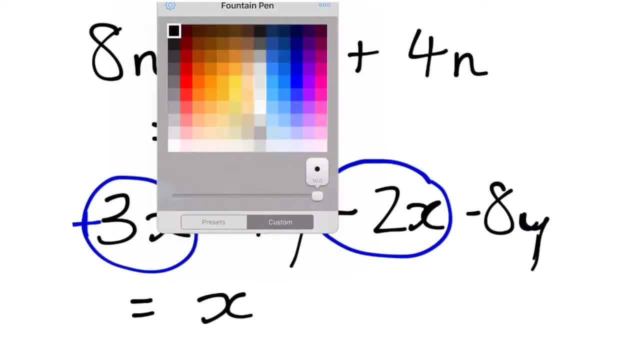 2x will be 1x, And when we've got one lot of x, we just write x, We don't write the 1 in front of it. And then for the y's I need to combine those as well. I'll circle. 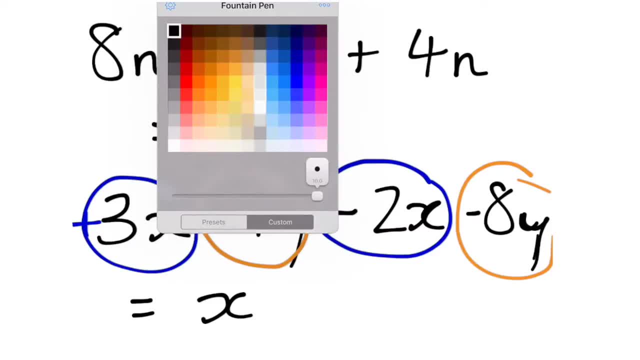 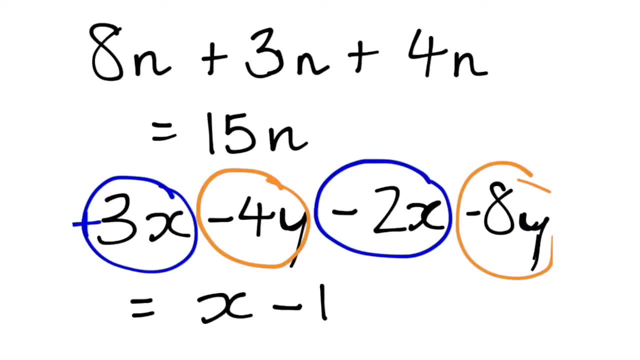 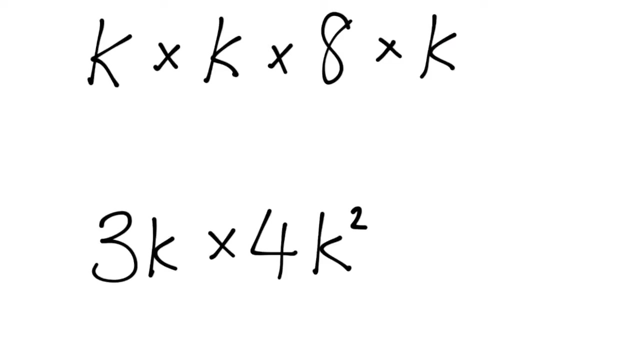 them including the sign Minus 4y, minus 8y. Minus 4 minus 8 is minus 12, lots of y. So there are two examples of simplifying terms with addition and subtraction. We can also simplify expressions with multiplication. So in this first example I've got k times. 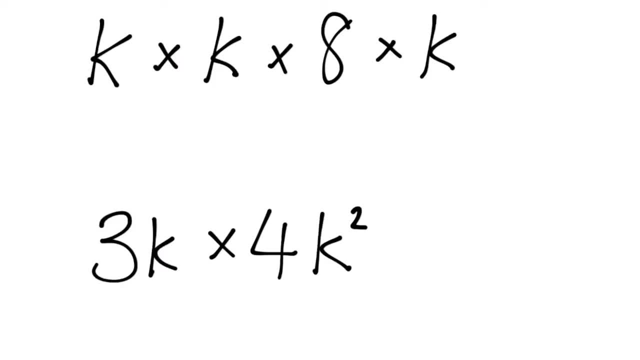 k times k, 8 times k. Now, an easier way of writing k times k times k. well, think about 3 times 3.. What's an easier way of writing 3 times 3? Is 3 squared, So k times k times. 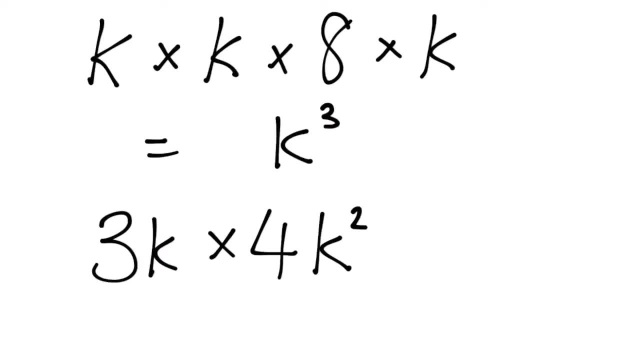 k will be 8, sorry, k cubed. All right, that's another way of writing repeated multiplication. and because I've also got the 8 there, I've got 8. lots of k cubed. Okay, for this second. 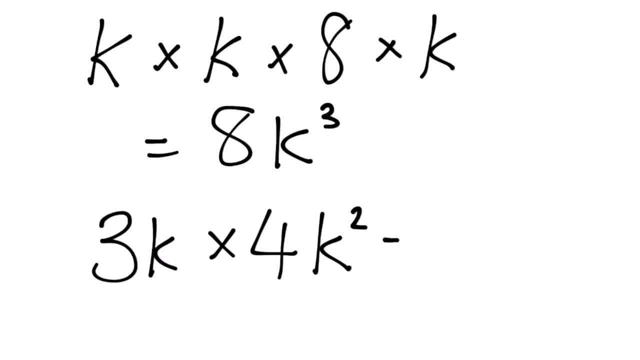 one. I've got 3k times 4k squared. you need to treat these as numbers and letters, So first look at the numbers. You've got 3 times k times 4k squared. 3k times 4k squared. 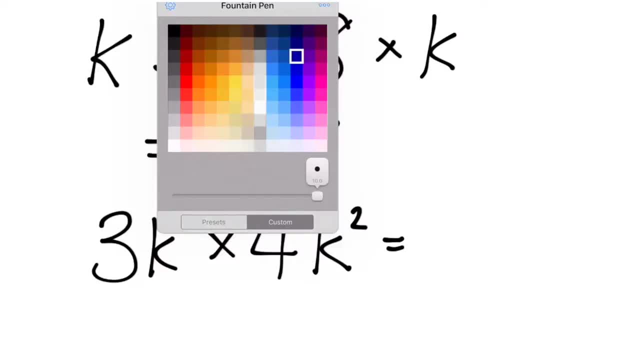 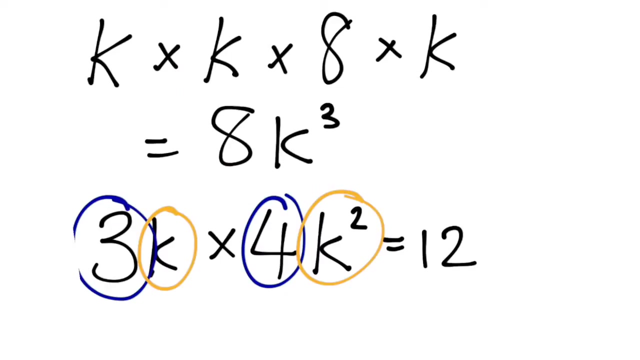 four. You could almost think about this as two separate operations. First, do the numbers three times four, twelve. then do the k's, So k times k squared. What's k times k squared? That's the same as saying k times k times k k, cubed, If you know your. 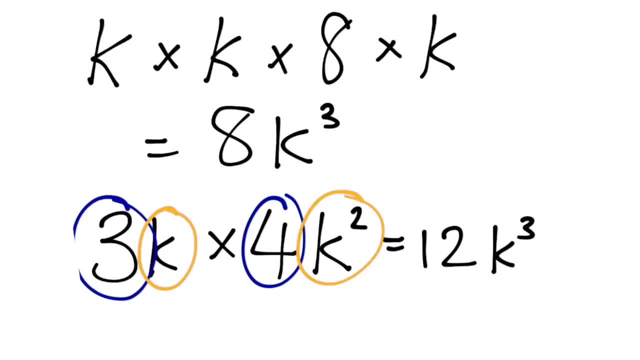 indices laws. you know that you can add the indices. that will give you k cubed as well. So twelve k cubed is the answer to that one. So that's an example of simplifying expressions with multiplication signs in them. That's one of the rules of simplifying expressions. 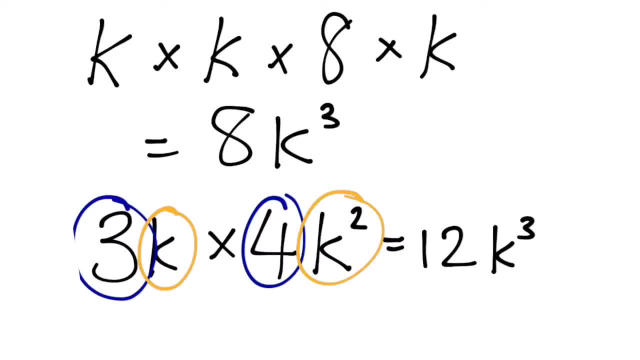 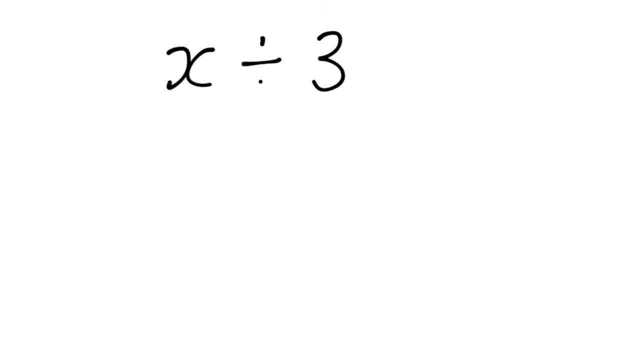 We never write a multiplication sign in an expression. An expression in its simplest form won't have any multiplication signs. When we're simplifying expressions and we see a divide sign, you need to remember that you write those as a fraction like that. While you might think that's not any simpler, that's just the convention. 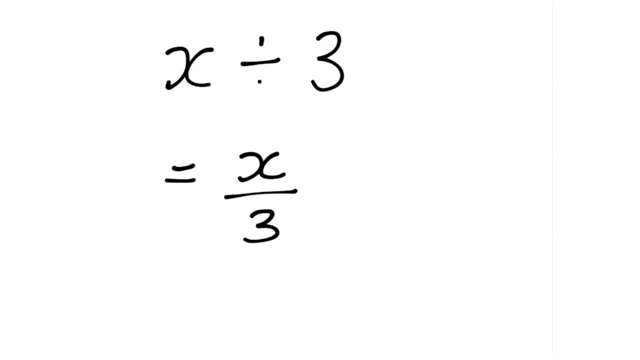 and that's something you'll need to get used to. It makes things easier down the road. Okay, so let's look at some expressions with a combination of additions and multiplications, divisions and subtractions. The first example here is three r plus three times two r. What's? 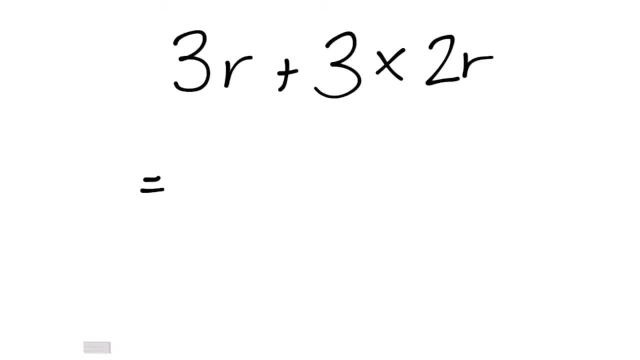 the trick you have to remember here: R, big maths right. Do the multiplication before you do the addition. So three times two r, three times two r first. So leave that addition until last. We need to do three times two r, that's six r, Then we've got three lots. 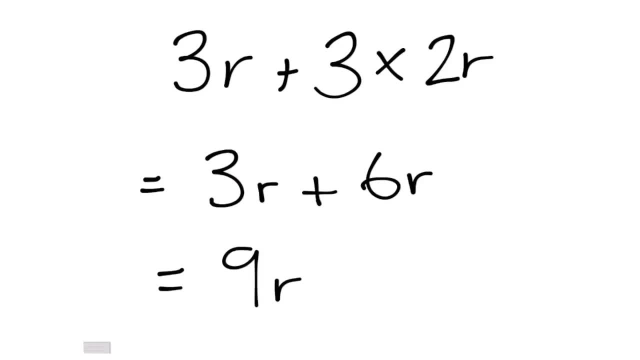 of r plus six r, nine r. Okay, next example: six x divided by two plus x. What do you have to remember? Big maths Order of operations: the division comes first. So six x divided by two, three x, Then I've got that plus x. Are these like terms? No, they're not, They're. 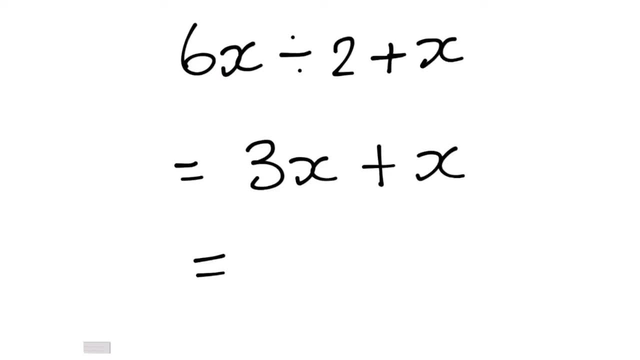 terms? Yes, they are, So I can combine them: Three x plus x, or one x four, lots of x. That's your final answer. Okay, so we've done how to add, how to subtract. we've done multiplication. 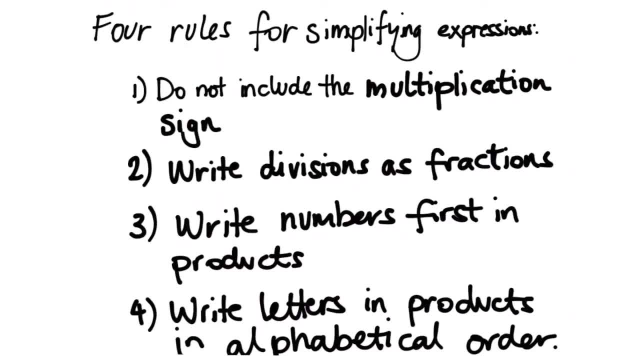 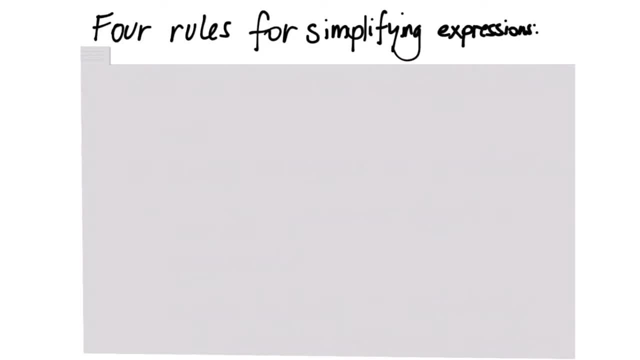 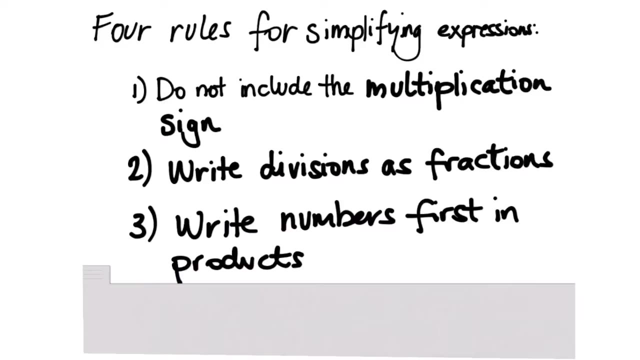 division, and then we've combined them all together And now I want to give you four rules to help you remember this process. Four rules of simplifying expressions. Do not include the multiplication sign. Write divisions as fractions in your answers. Write numbers first in products. What does that? 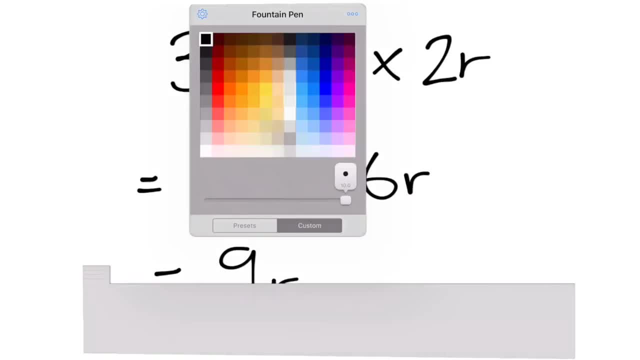 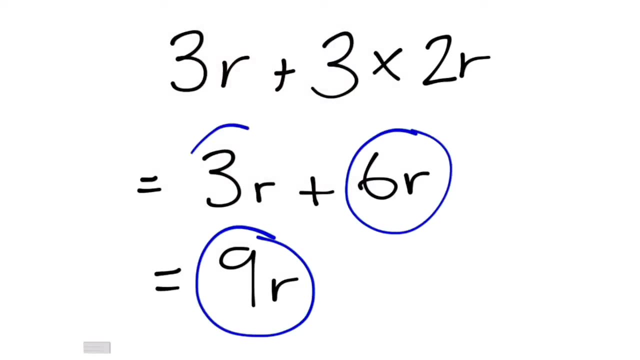 mean: Well, for example, this is a product, this is a product, this is a product. We always write the number before the letters. Okay, so the number comes first in any product, And so write numbers first in products. and 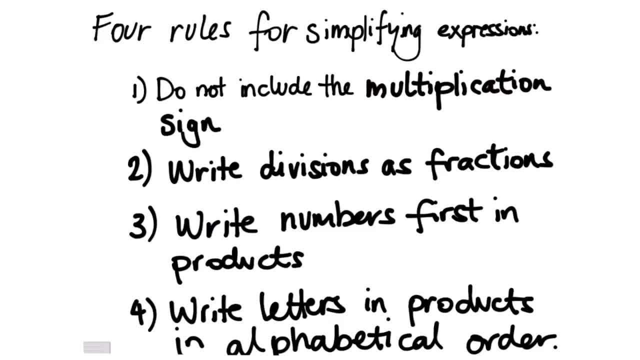 the last one write letters in products in alphabetical order. So if you had something like six x a- x b, you wouldn't write that as six b a, you'd write it as six a- b. So the letters should come in alphabetical order. Okay, I hope this video has been helpful for. 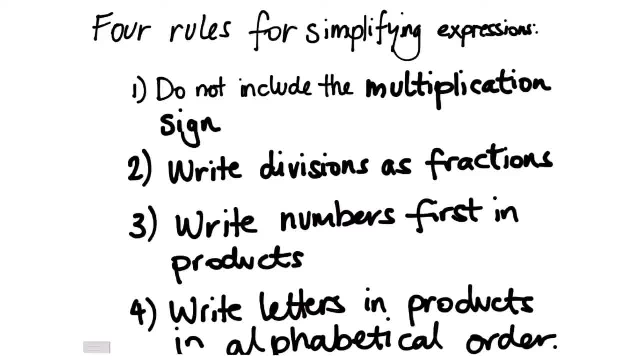 you when you're simplifying expressions. I think if you can try to remember these four rules, check out my examples and you should master those pretty quickly. Thanks for watching. I'll see you in the next video. Bye.